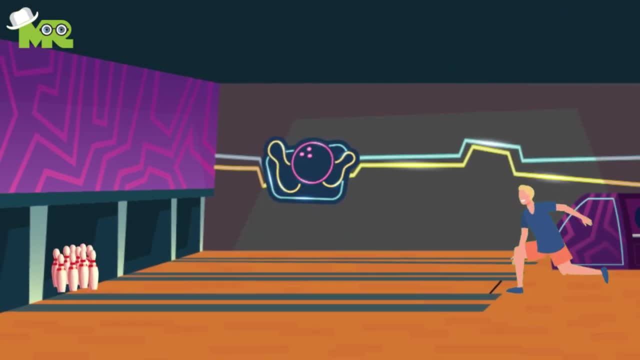 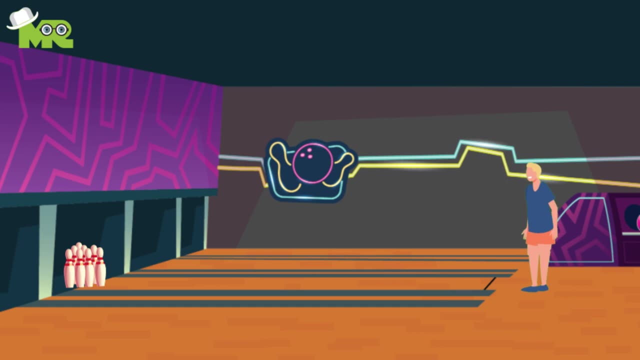 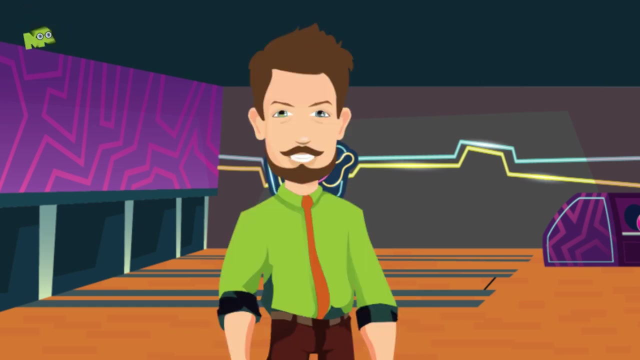 that frame Three. in case a player knocks down nine pins with the first shot but misses with the second, the player will still score nine points. Four players are awarded bonus points for strike and spare Five. an average of three games is played. A three-game average is determined. 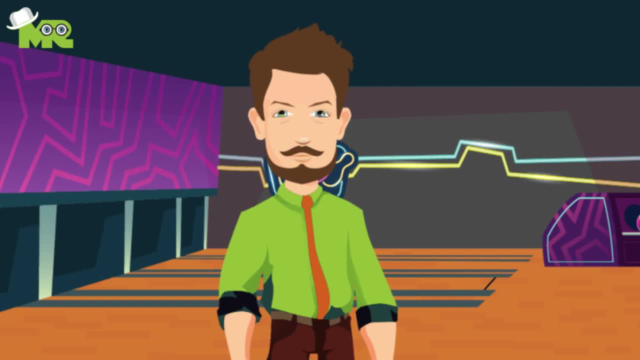 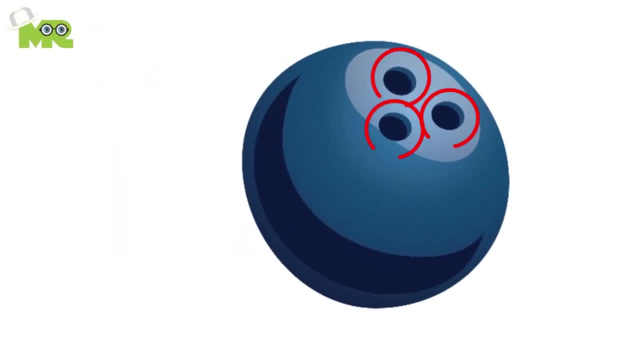 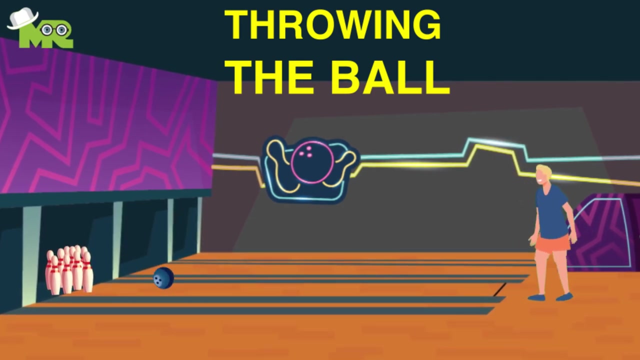 by adding all three scores and then dividing that number by three Rules of bowling. One: it is necessary for the players to hold the ball using the three-finger drilled holes on the ball. Two: each frame consists of throwing the ball twice to knock down all the. 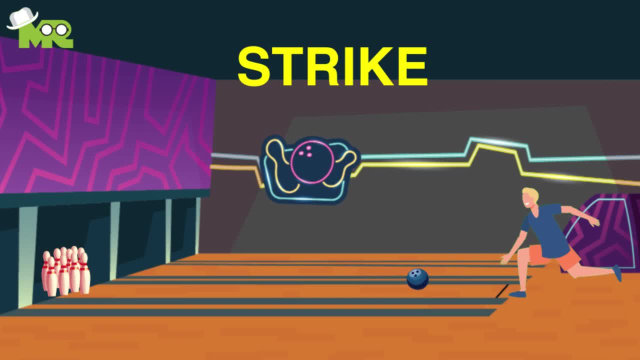 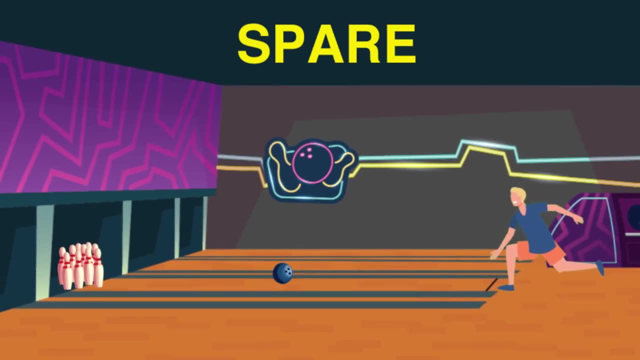 pins. Three: it is called a strike if you knock down all the pins with the first of the throw of the balls. Four: it is called a spare if you knock down all the pins with the second ball. Five: each game consists of 10 frames. If you bowl a strike, 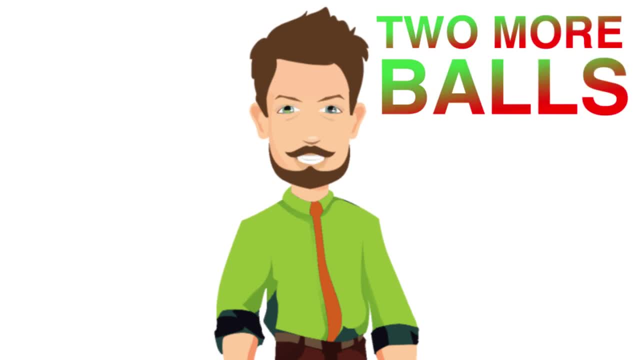 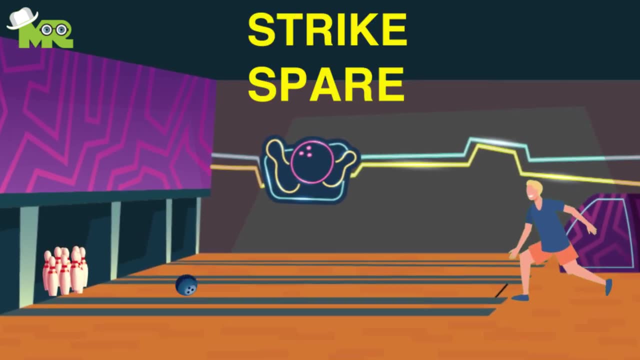 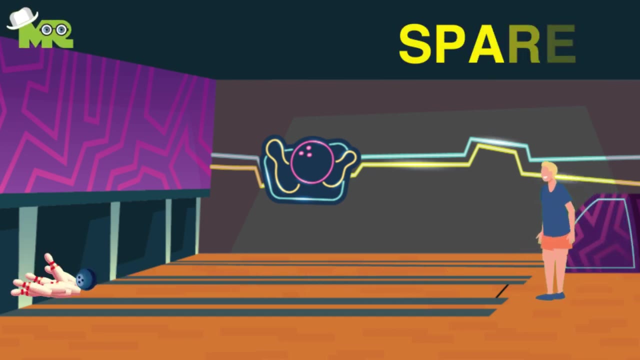 in the 10th frame, you get two more balls. If you throw a spare, you get one more ball. Six: if a frame doesn't have a strike or a spare, it's known as open. Seven: you get to add the pins in your next ball to that frame if you bowl a spare. 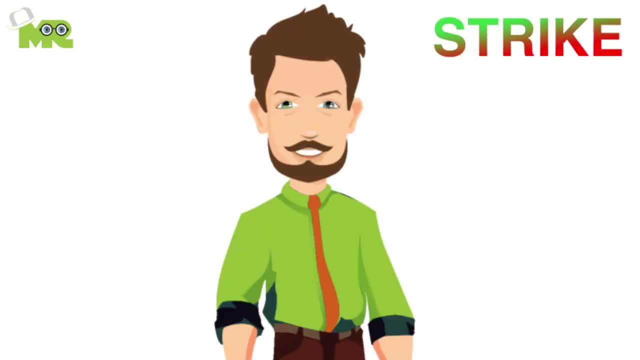 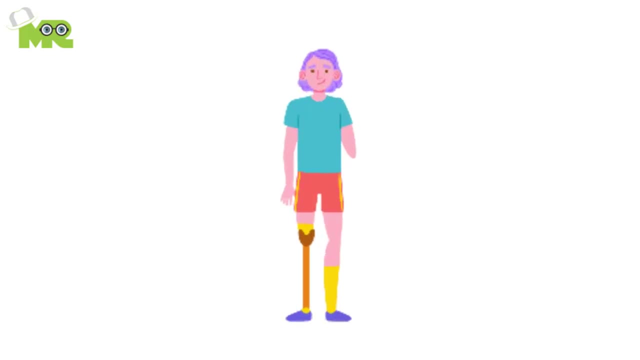 You get to add the next two balls if you throw a strike. Eight: if you step over the foul line, any pins knocked down will not count towards your score. Nine: if the athletes are not able to score, you get to add the pins in your next ball. 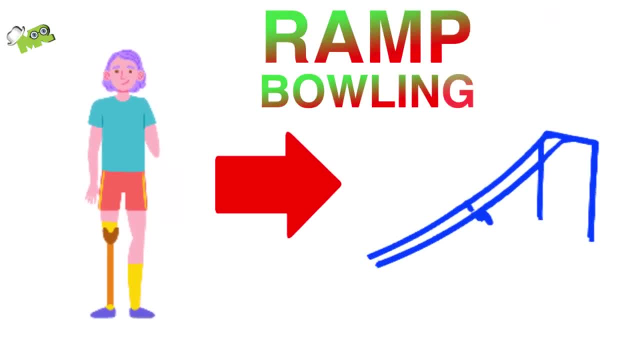 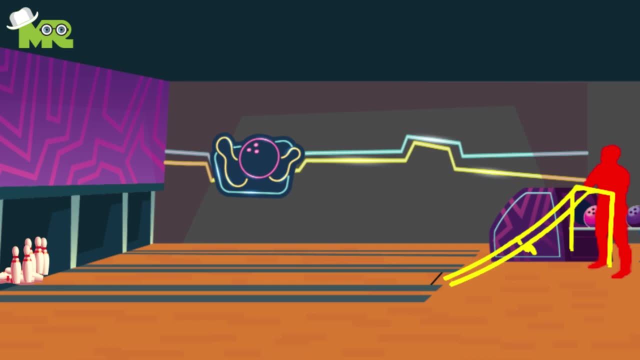 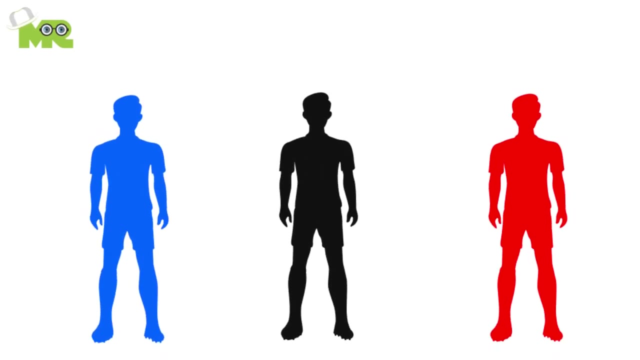 Ten: if a player is not physically capable of rolling a bowling ball ramp, bowling is allowed. The ramp is strictly for physical disabilities and cannot be used just to improve the scores. Ten: bumpers are not allowed while bowling professionally. Eleven: if the game has more than one bowler, every bowler will take their frame in a 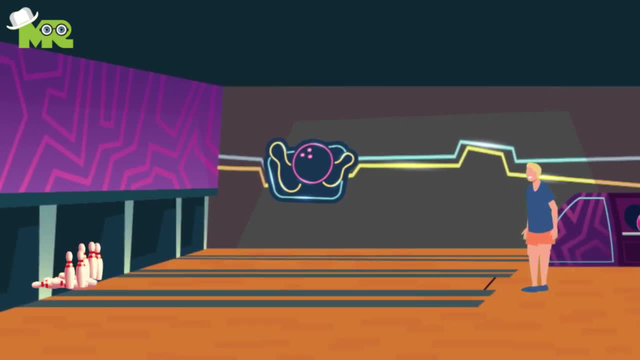 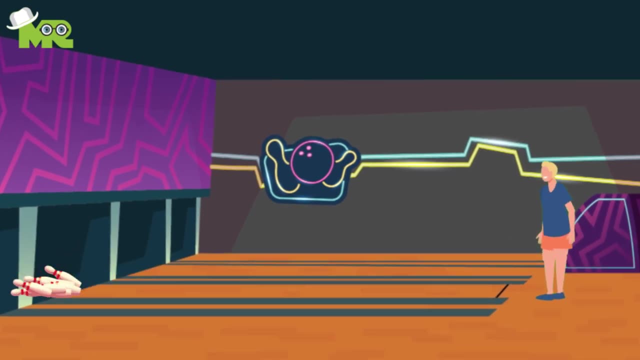 predetermined order before the next frame begins. Twelve: in case the bowler knocks down all 10 pins in the 10th frame, the bowler is allowed to throw three balls for that frame. This allows for a potential of 12 strikes in a single game and a maximum score of 300 points. 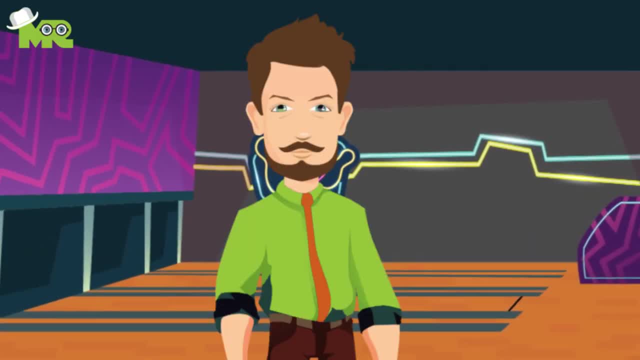 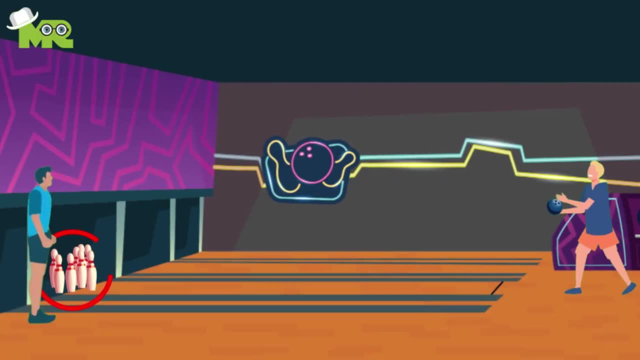 Thirteen: in the case of a dead ball, the chance is not counted and the player is given another chance to bowl. The ball is considered dead under the following cases: One, if the player notices that some of the pins are missing from the setup while delivering the ball. Two, in case a human.